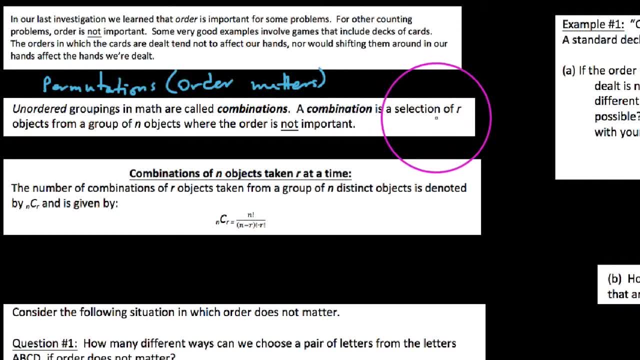 permutations. we say: order matters, okay, Permutated groupings, permutations, permuted groupings, order matters. we say a combination really is saying we want to select r things from a group of n total things, but order is not important here, okay. So that being said, 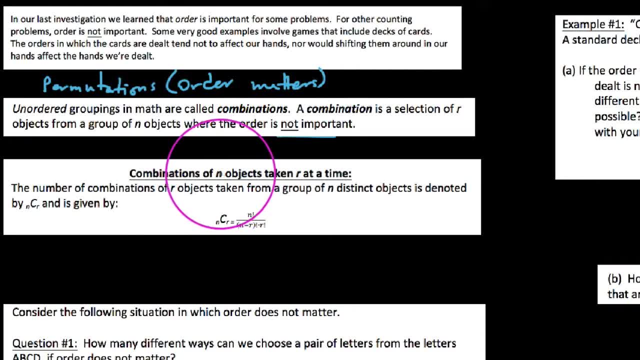 let's go ahead and take a look at our expression here. that allows us to calculate if we have n total things- and I want to select groups of r of those things at a time, how we actually do this here- and it says the number of combinations of r objects taken from a group of n distinct objects. 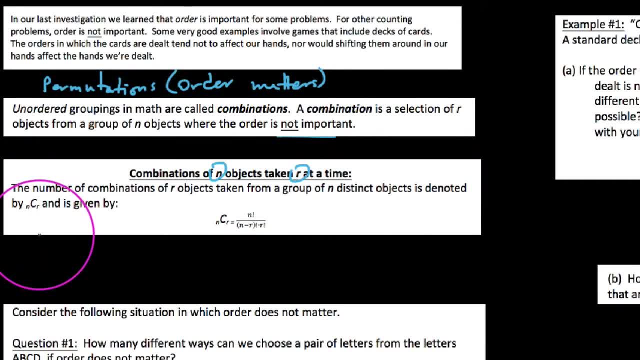 is denoted by n, with these little subscripts. here we have n choosing r and we would- let's write it this way- we say n choose r, with these subscripts where n represents the total number of objects that you have to begin with. so I'm going to make a little note here. this is the. 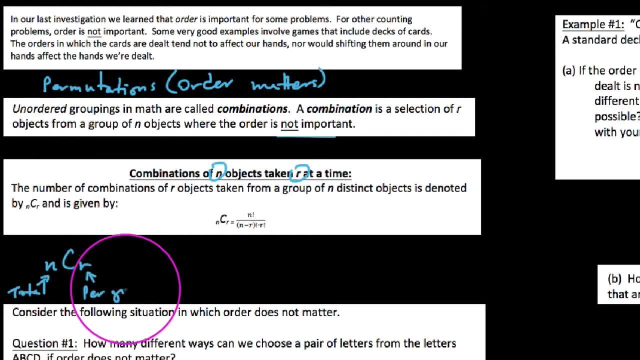 total and this is the number per group that you want. okay, This is how many of those n you want to select at a time, and we say that. the formula for this, just to make this a little bit clearer. here we say n choosing r at a time, which, by the way you'll sometimes see, is written in: 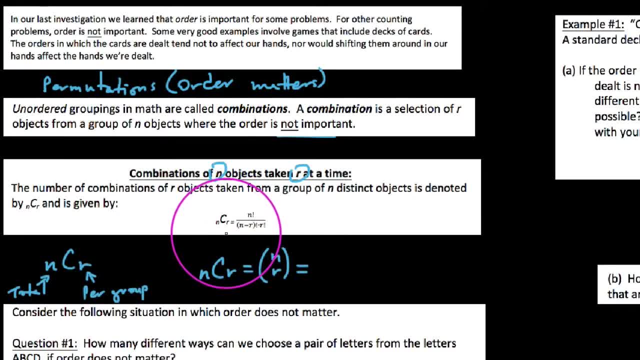 parentheses like this: n choose r, and that's how you read it. n things choosing r at a time. we say is n factorial and it'll be over: r factorial, n minus r factorial, and this is supposed to be a parenthesis here, but essentially what I want. 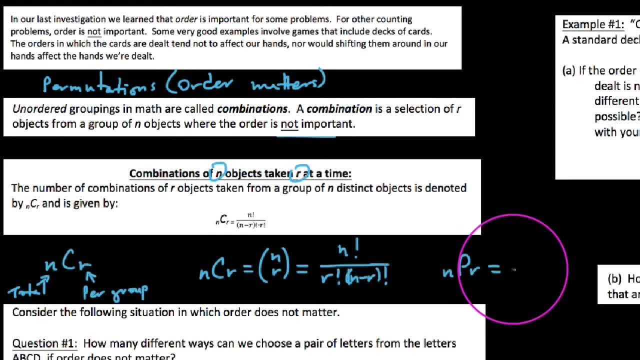 everybody to see here is this: when you look at permutations, which order does matter? we said it has an expression as well. we say n things rearranging r at a time that was n factorial over n minus r, that quantity factorial. so what I want everybody to see here is really the only. 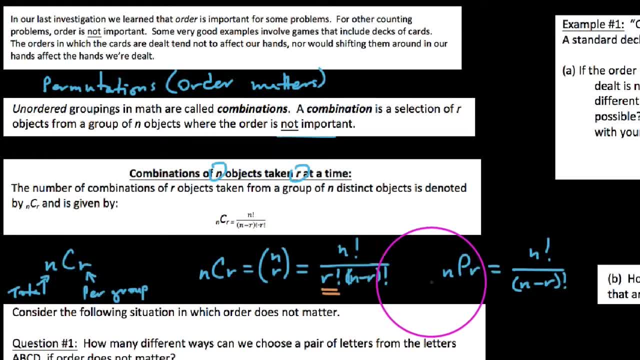 difference between combinations and permutations is that there is an additional factor in the denominator of a combination, and that additional factor is this r, right here, this r value, okay, remembering that r represents how many things you're choosing at a time. so, to kind of confront why this works the way it does, what I want to do is I want to kind of consider: 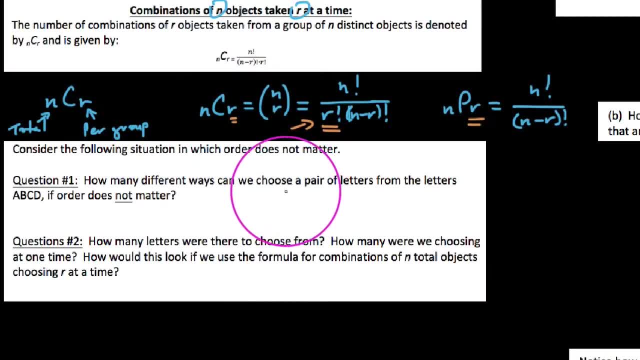 this thought experiment here, but it says how many different ways could we choose a pair, so two letters at a time, from the letters a, b, c, d, if order does not matter, and I think that in this instance it's actually beneficial to write these pairs out so we could say well, 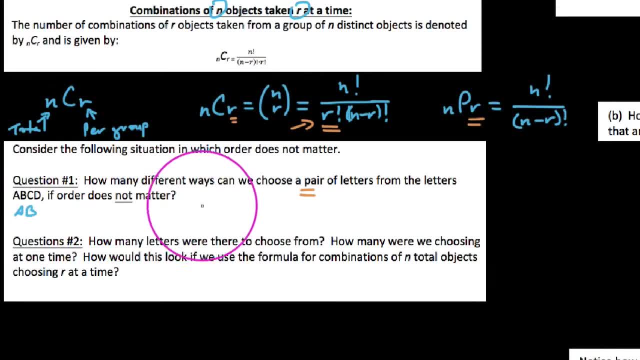 there's a- b, that would be one pair, and if order doesn't matter, what I want you to see is we would not say that b a is any different from this, because if order doesn't matter, these really truly matter. 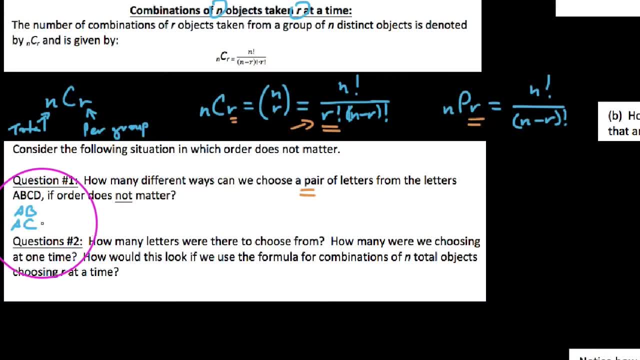 They mean the same thing. so we say a b. that's already selected. we could say a c. we could also say a d. so now I've paired everything with a. we could say also b c. we could also say b d. 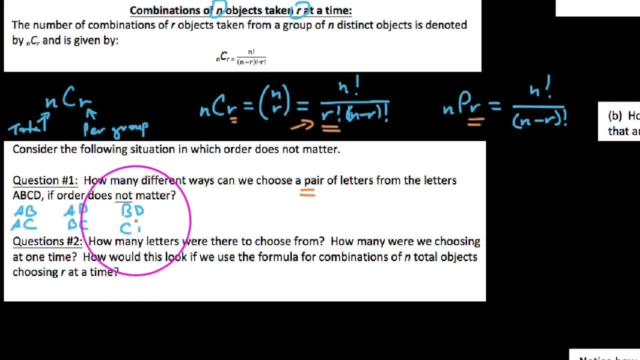 now I've paired everything with b, we could say that the last possible combination would be c- d. so in terms of how many ways there exists to do this, then we would say that there are six outcomes in terms of selecting two letters or a pair of letters from four letters, if order. 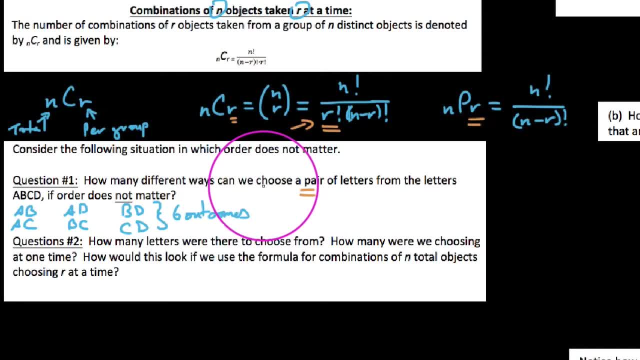 doesn't matter. Now I want everybody to consider this. If we've been discussing permutations, that is, you know, I have four total letters. how many different ways could you choose two? if order did matter? and what I could have, you see, is this: we would also have to have b? a. with a b, we could. 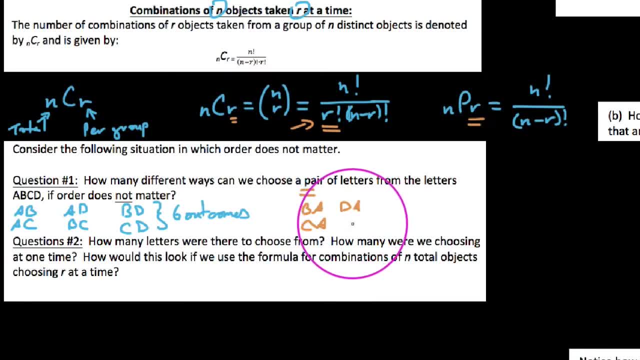 say c a also needed d a, we would need c b- I'm just flipping all those around- we would say d b and we'd also say d c. so not only would we have all of these over here, we'd have to have these. 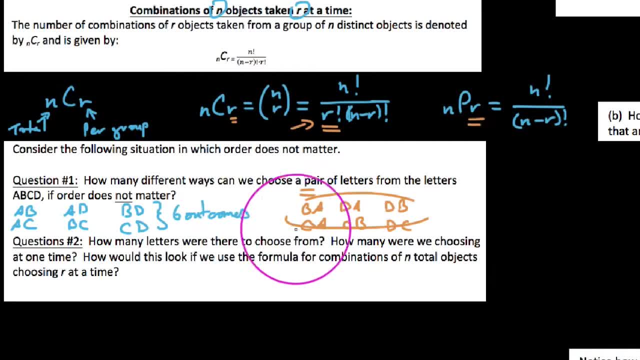 also because we'd have to rearrange them. but what we're kind of saying here is this: with combinations, we don't have to worry about the rearrangements. so one thing I'll tell you is this, in terms of combinations- since order does not matter- 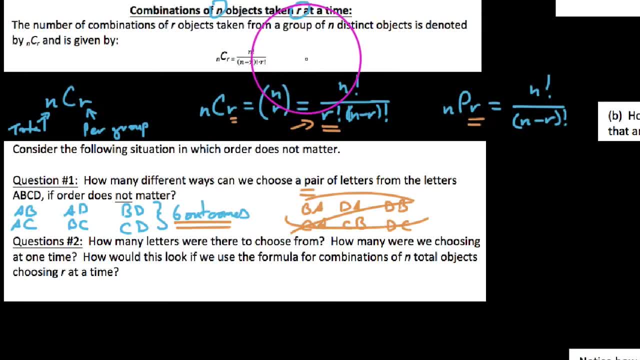 there will always be fewer combinations than there will be permutations. so there- I don't want to say always, but almost all of the time- there are fewer combos than permutations. okay, because order doesn't matter, you can knock out all the ones in which you switch the order around, because you 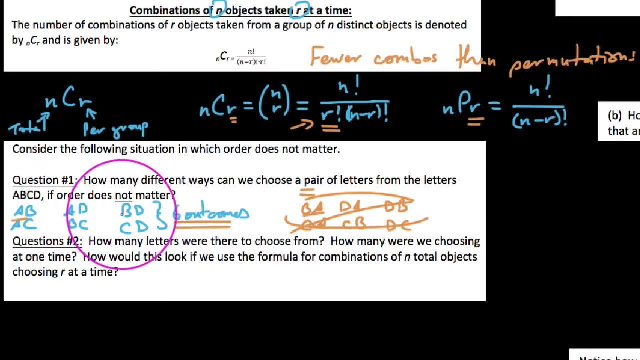 know they count as the same thing, as if order didn't matter. they count as the same thing as their other pair. anyways, in this case, another pair, and then also this: we say: well, I don't know if I had these six combinations in the first place and I rearranged them, how many? 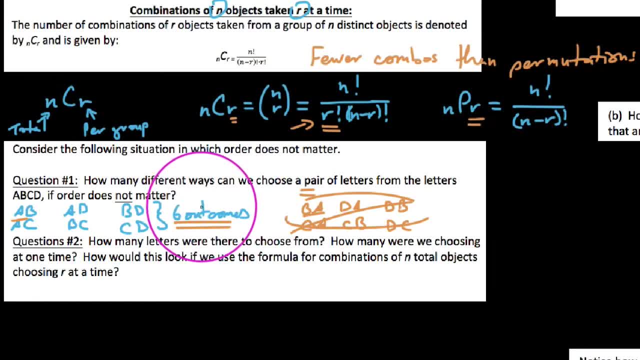 exist to rearrange two letters where there are two factorial ways to do it. so what we could have said was this: we could have found four permute two. we could have said: well, four permuting two. that would be how many ways you could do this, if order did matter. but what I'm saying is the thing. 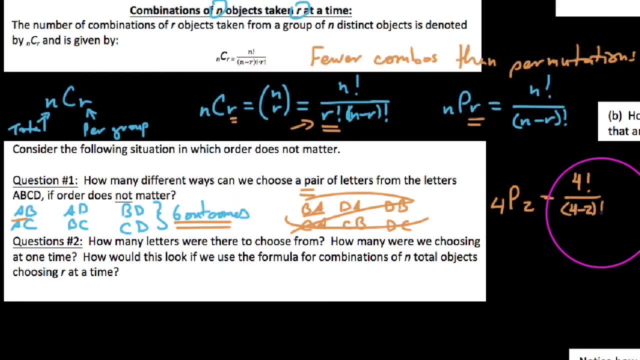 that makes this a little bit different from a combination. is this a permutation order matters. with a combination, we said, well, now, if I just want just these. what we'll do is we'll divide out all of the repeaters and in this case we say that there are, since two, there are two. 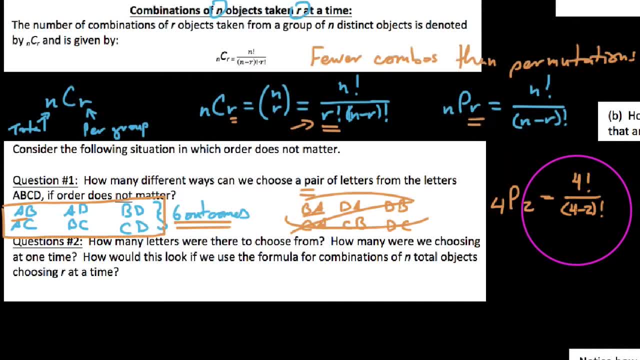 letters. how many ways exist to rearrange the two letters? there are two factorial ways to do it. we have to divide out an extra two factorial and so I hope everybody sees this here. if I do that, then what that does is it mystically transforms this into saying: well, if we divide out all the 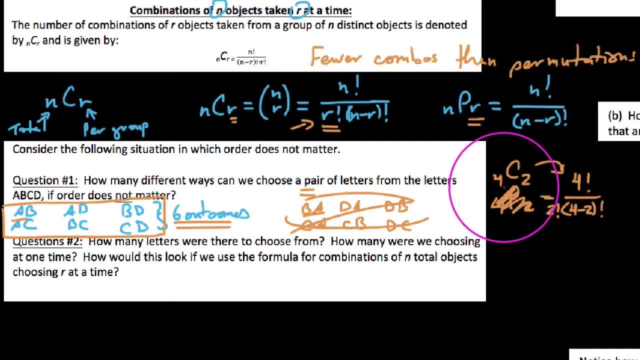 repeaters. now we're talking about a combination, and what you see right here really is this: our n would be four, our r is two, and if we were to use the expression now for n, choosing r at a time where order doesn't matter, we could have said it would have been n factorial or four factorial. 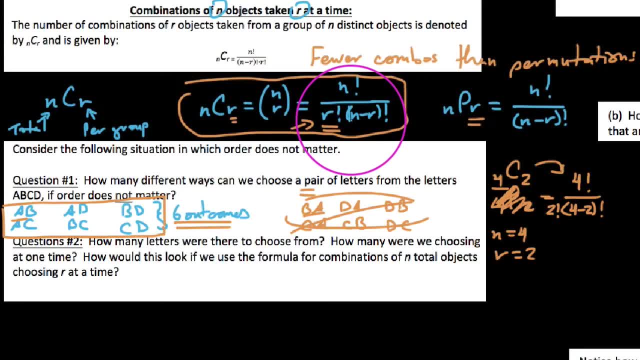 that's our n value here Over r factorial: n minus r factorial, where we say r. well, r in this instance is two, so we get two factorial times four minus two factorial. So by writing all of these out, we were able to determine that there were six possible ways. 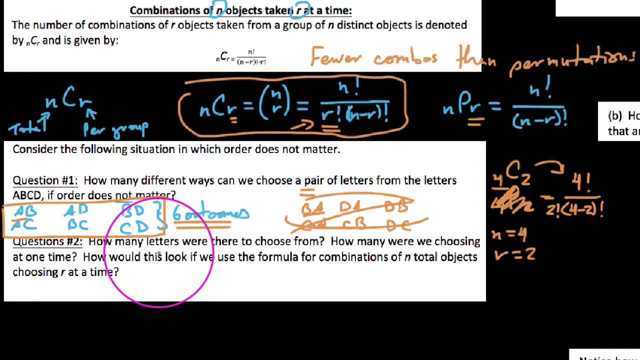 to get two things from four things, if order doesn't matter. what I want to know now is this: how many letters were there to choose from? we said that there are four letters to choose from. we say: how many were we choosing at one time? this is going to represent our r value. 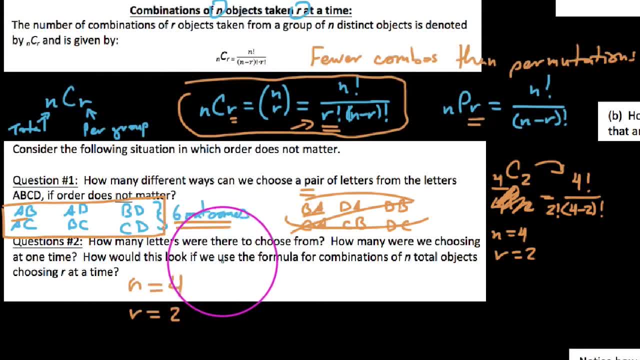 we say: well, I was choosing groups of two at a time. it says: how would this look if we used the formula for combinations of n and r? So we have n total objects choosing r of those objects at a time. and so again we could say: 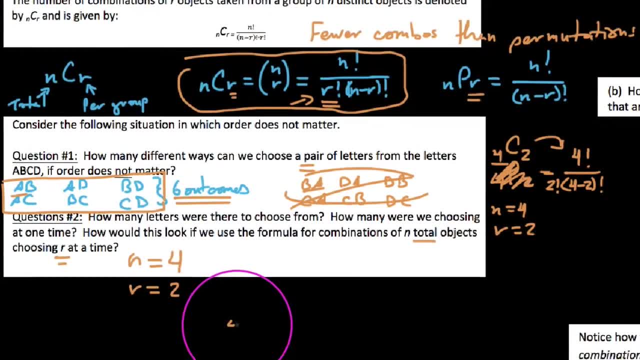 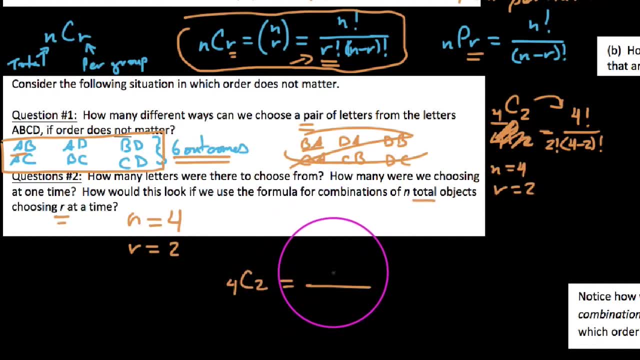 well, if order doesn't matter, here I've got four total objects. I want to know how many ways, if I have four things, that I could choose just two out of that group at a time. how many groups of two could you make if order doesn't matter? and again we could say: 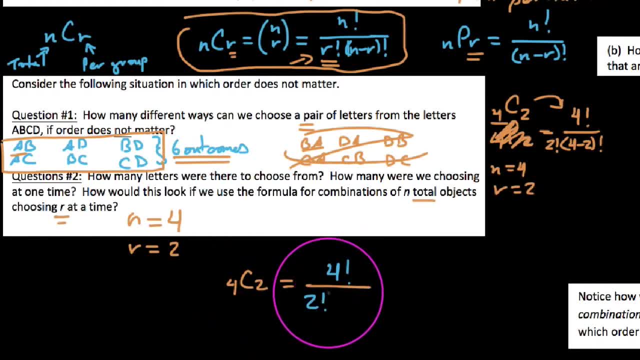 well, it's four factorial over r factorial. so we say r is two and this would be, you know, times four minus two factorial. so we need to simplify this and what we end up with here is this: we say four factorial over two factorial, times two factorial, and again. 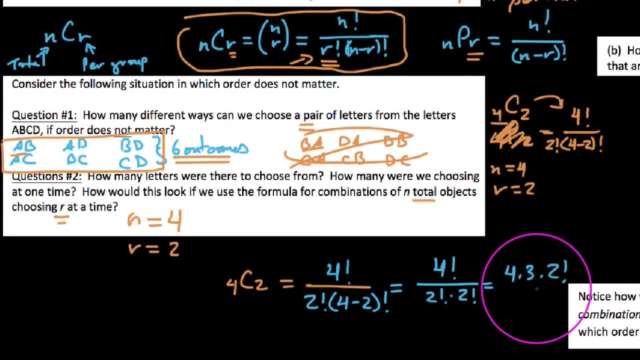 know simplifying this. we can say that's 4 times 3 times 2 factorial, over 2 factorial times 2 factorial, and we could at least cut out one of these twos factorial and we get this. we get 4 times 3 on top, which is 12, and then we say on the basement, here in the denominator, we say 2. 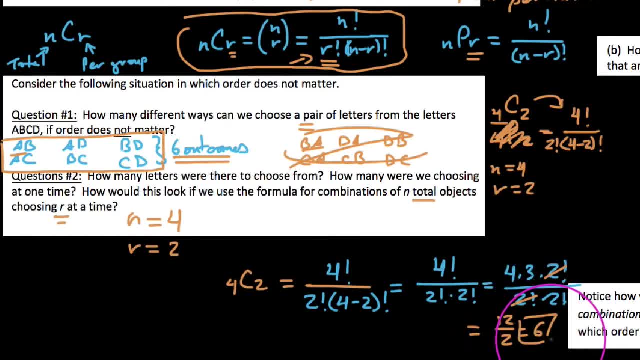 factorial, which is 2 times 1, we just get 2. so, in other words, here are our six outcomes that we were able to determine by writing it all out here. but what I want you to see is that, not in all instances where you have four things and only choose two and be able to write them all out, we're going to 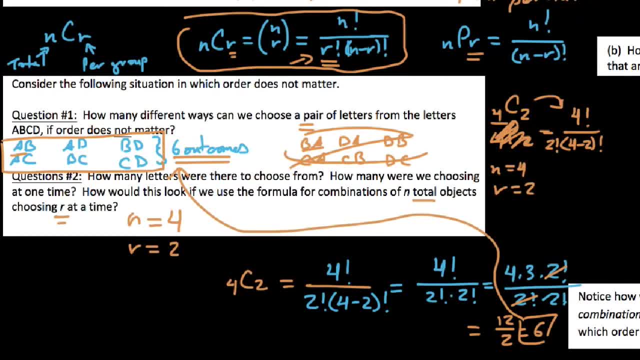 have immense numbers of outcomes. so we're going to do for the remainder of this video is we're going to tie this into the fundamental counting principle as well as look at situations in which the number of combinations is so immense that you couldn't necessarily do this by scribbling. 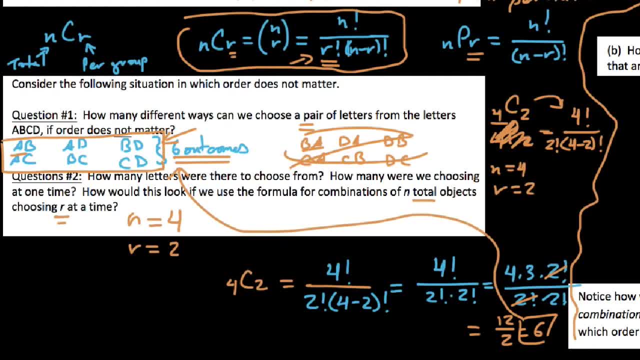 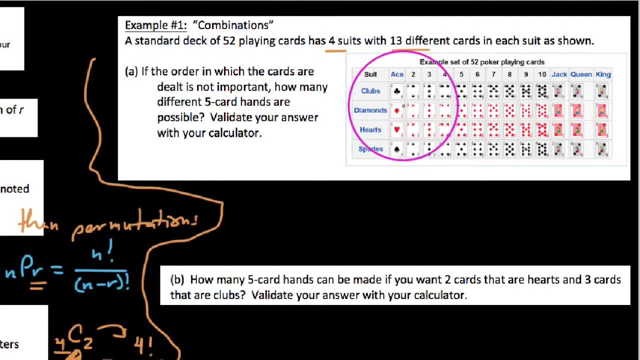 out all the possibilities, you're going to have to use your combinations formula. so let's go ahead and consider a deck of cards here. we say a standard deck of 52 playing cards has four suits with 13 different cards. you know, we say four suits: clubs, diamonds, hearts, spades- we say 13. 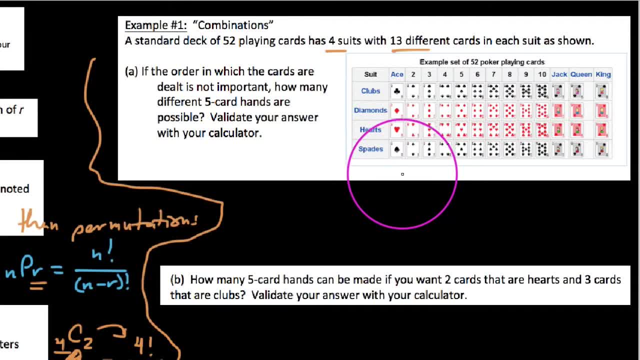 different kinds of card pursuits. so four times 13, this is our standard deck of total 52 cards. we have a total of 52 cards. what I want to know is this: if the order in which the cards is dealt is not important to the order in which you hold them, is not? 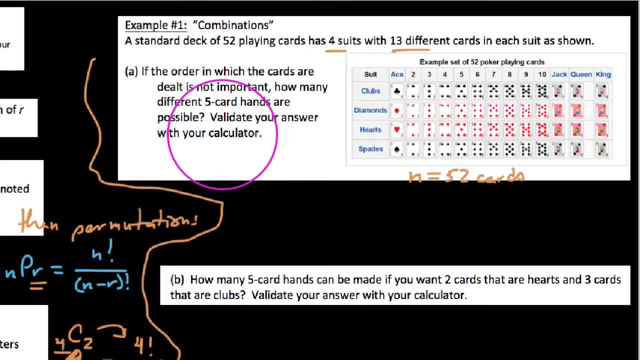 important, how many different five card hands could we have possible? and so what we're going to do is this. we're going to say: well, if I had 52 total things and I want to choose groups of five at a time, so our r-value is five- we would say that, in the total number of ways to do this would be 52. 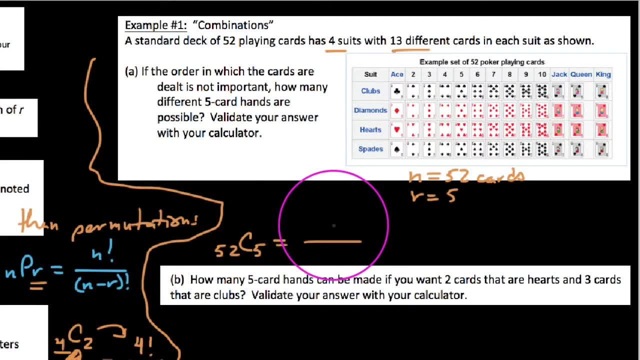 things, choosing groups of five at a time. we'll just go and drop this into our combinations formula, and so we get this. we say, well, 52 total things, 52 factorial, and this would be over r factorial. so five factorial times 52 minus five factorial and, again simplifying this, I get 52 factorial. 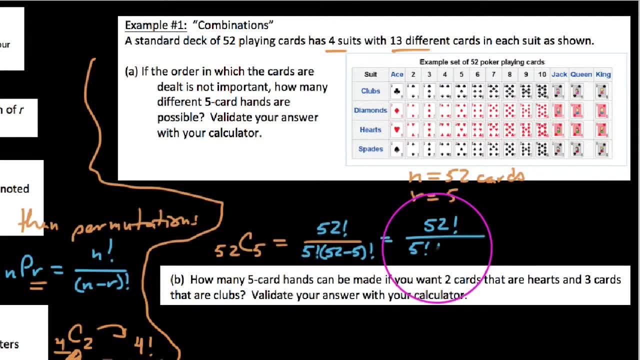 this would be over five factorial times, 47 factorial, and you know what. writing this out. actually, I do want to take the time to write this out now. most calculators have a combinations function on it. unfortunately, the calculator that I have available to me does not, so I'm going to. 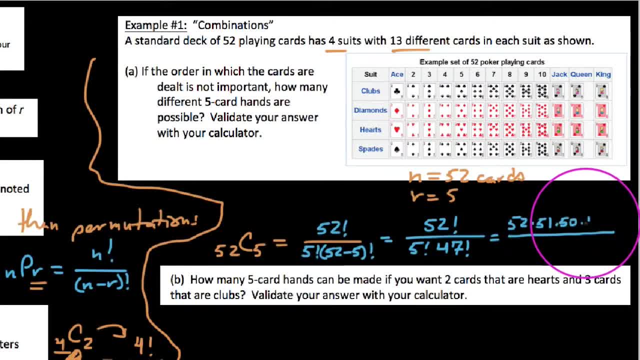 write out a few terms here: 52 times 51 times 50 times 49 times 48- I'm going to squeeze this in here- times 47 factorial, and this is all over five factorial. times 47 factorial. okay, so I'm going to cross out the 47 factorial and what I'm. 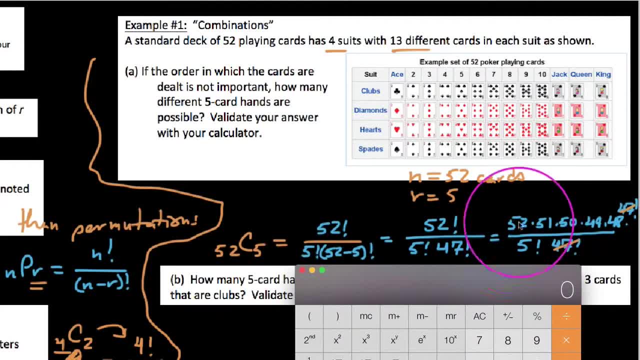 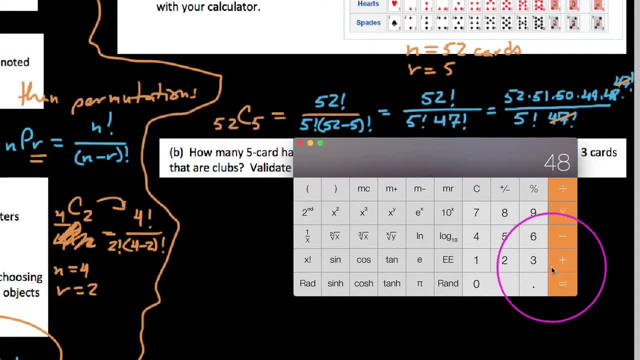 going to need to do now is grab my calculator and I'm going to get an expression on the top here. so we say 52 times 51 times, 50 times 49 times 48. so we get this number here and I'll add that to my 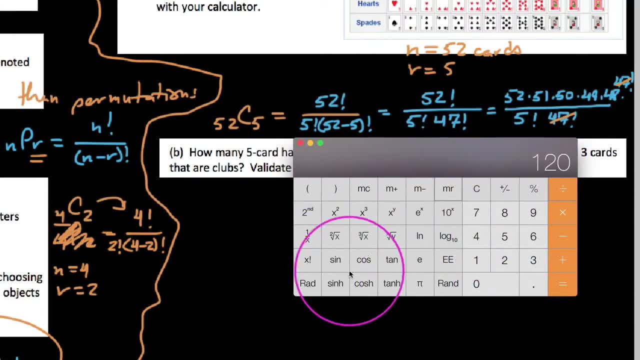 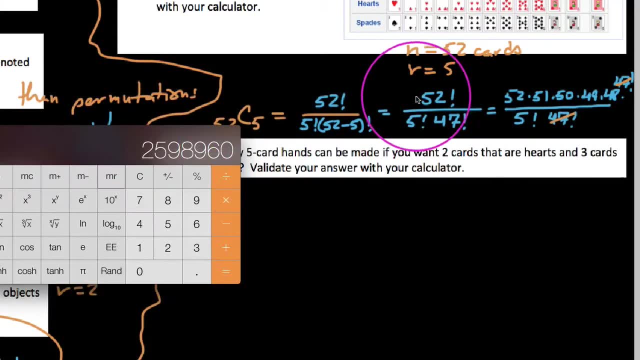 memory there, memory plus, and we're going to divide that by the number here and we're going to divide that by five factorial, and what we end up with is this: so the number of five card hands you can make- if order doesn't matter- is two five, nine eight, nine six, zero. so we'd say equals two five, nine eight. 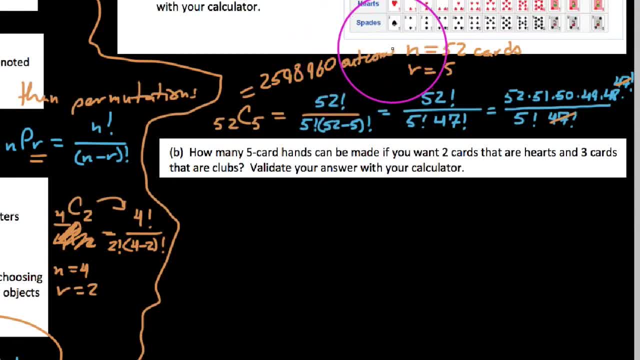 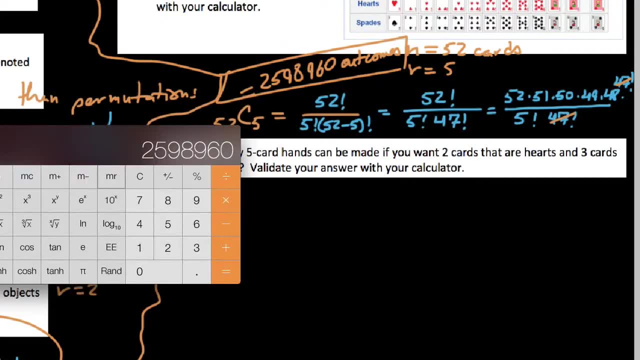 nine, six, zero, and that kind of makes sense that there are this many different five card hand outcomes, because there's quite a few to choose from in the first place. now, one thing I do want to tell you is this: if your calculator- and actually this one probably would do it, we could. 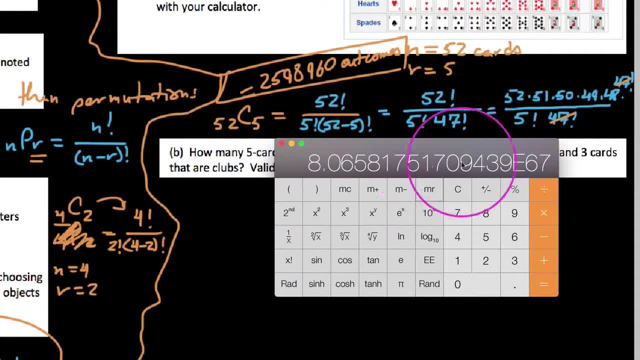 have typed this in as as this. we could have said 52 factorial. just don't want to break my calculator that it gives it to us in scientific notation: eight point oh seven ish times 10 to the 67th. but we could have taken that and divided by now in parentheses, we could have said five factorial. 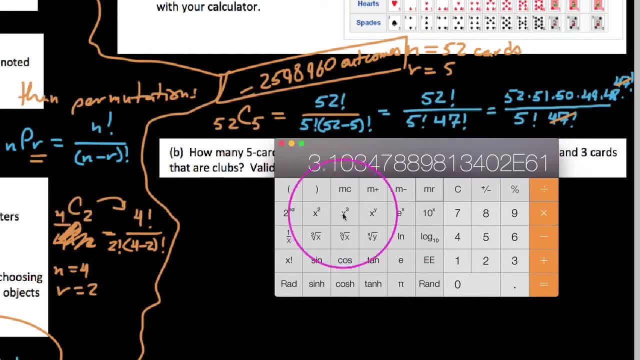 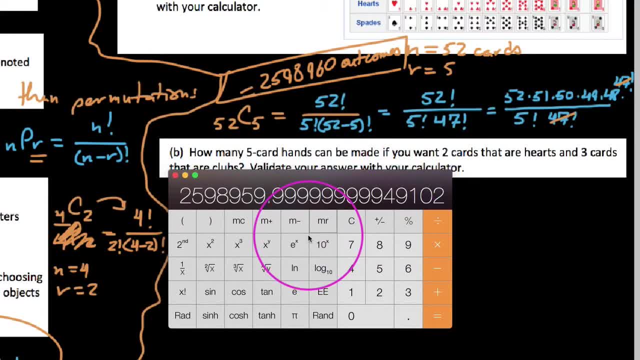 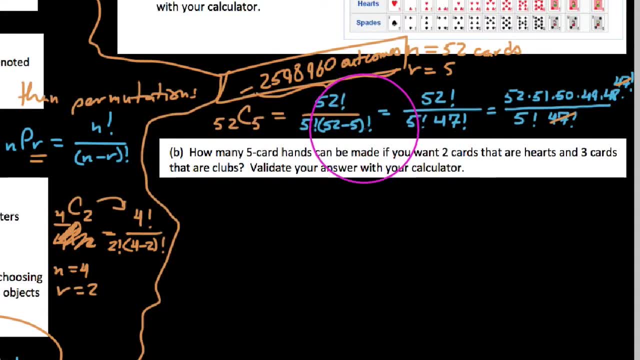 this problem here, because my calculator isn't equipped to do these. often. you see that I would have to kind of round this off. of course, there are only an integer value number of outcomes, because, well, you couldn't get a decimal number of hands with the five card deck. so 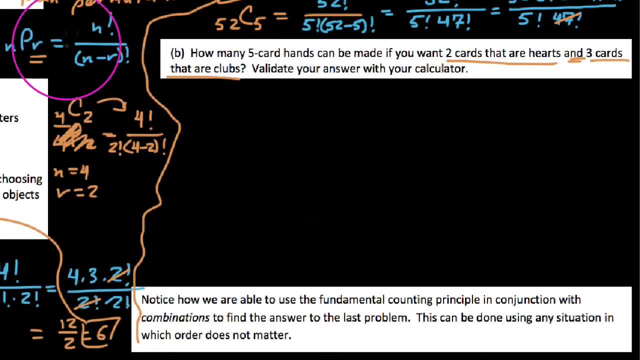 now, for example, what I want to do is I want to use our combination formula that we've been discussing here, where order doesn't matter, in conjunction with our fundamental counting principle or multiplication rule. okay, and remember, the multiplication rule says: if you want to find out the total number of ways to do a bunch of things in order, you know, like event one. 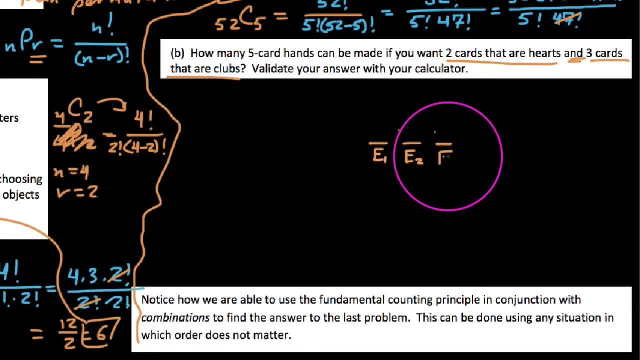 event two, event three, so on and so forth. the three. you know three things happening in order. you know n number of things happening in order. we say our nth event. if you want to define the total number of ways of doing this, we could just go through and find out how many ways exist to do each of these individual things and then just 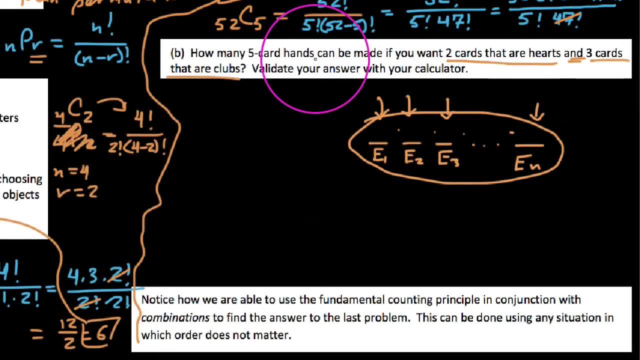 multiply them together. so reading through this is how many five card hands can be made. if we want to choose two cards that are hearts and three cards that are clubs, okay, and what we want to do is validate our answer with the calculator, well, i'll tell you what. in this instance, we have two. 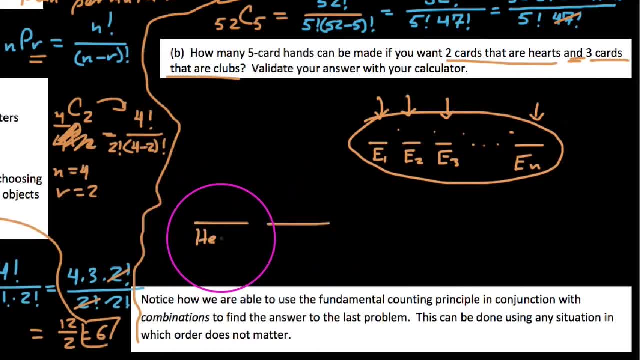 different events and so i'm going to put two different blanks down here. and just to be clear on this, we said two hearts, i wanted to choose two hearts, and i want to choose three clubs in my five card hand. so what we could do is we can consider this, we say all right, well, two cards that are 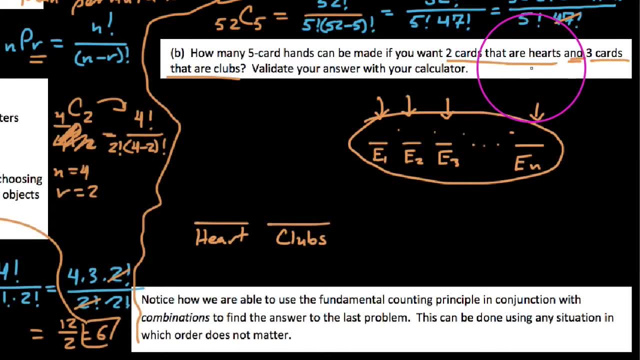 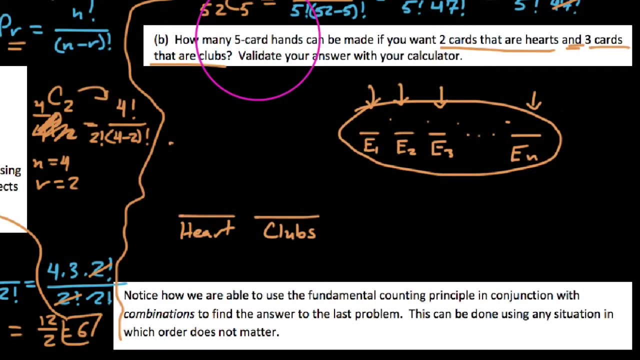 hearts. how many ways exist to get two cards that are hearts? and what we have to consider here is this: well, there are 13 total hearts in the deck, uh, so we would say, okay, if i just want two of them to be hearts, uh, for instance here. then what we'll do is we'll consider that, of the 13 hearts, we only 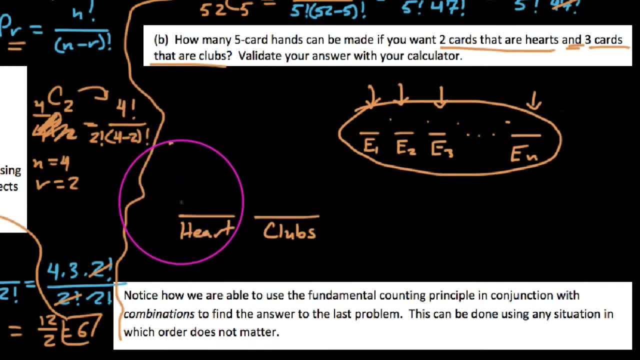 want to select two hearts of them. so how many ways exist to get two hearts from 13 hearts? we would say? well, 13 total things and i want to choose, you know, two at a time could be any two of those, but groups of two hearts at a. 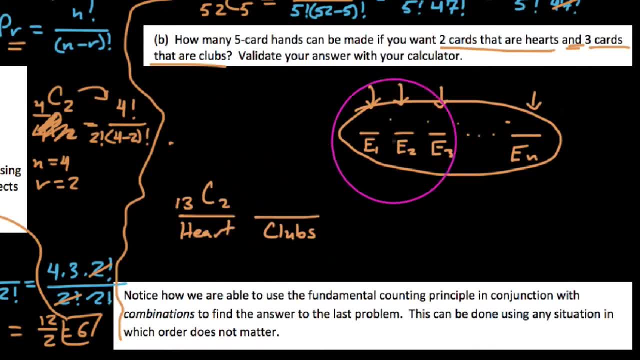 time. uh, now the fact is, you know, we say how many ways exist to choose three cards that are clubs. uh, there are also 13 clubs in the deck. okay, so we would say, of the 13 clubs, what i would like to do is choose three of those. so we say the way to do this, uh, in shorthand, rotation is just saying i. 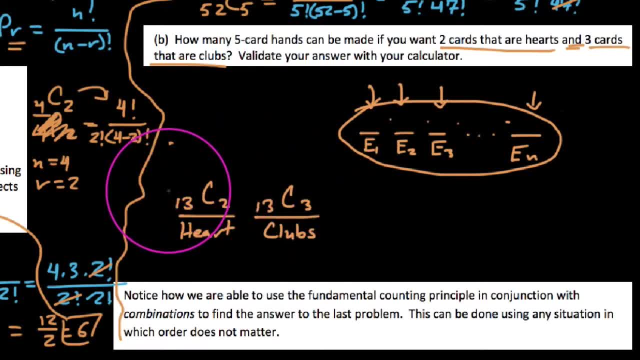 have 13 total clubs. how many groups of three could we make? the idea here is this: if i wanted to choose two hearts and, uh, three clubs, then we could say: let's find the number of ways to choose two hearts in the first place and find the number of ways of choosing three clubs, and then what we'll do. 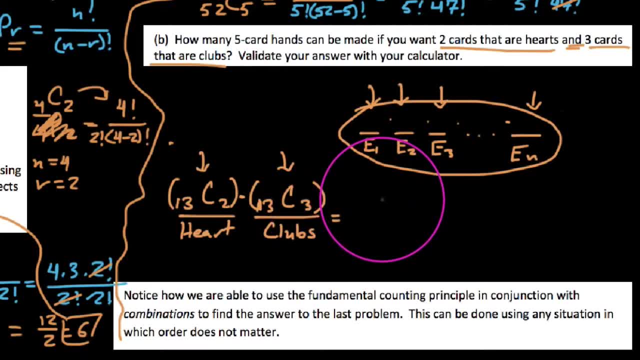 is, we'll just multiply these things out. so, going ahead and scribbling my work here, i would say that the first combination would be: 13 factorial over 2 factorial times 13 minus 2 factorial. we're going to take all of that right there. times now: 13 factorial. 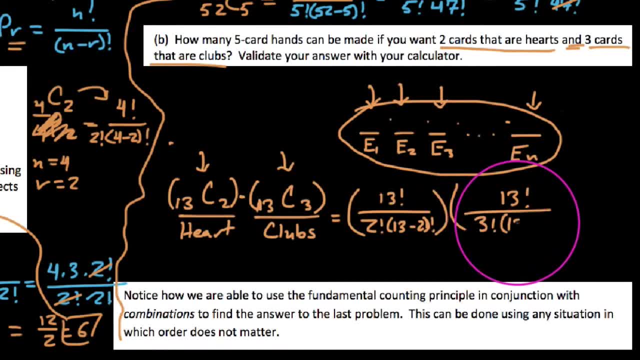 over- sorry, yes, over 3 factorial, 13 minus 3 factorial, all this, and so, in other words, we simplify this out to being 13 factorial over 2 factorial, 11 factorial, and then this one will be 13 factorial over 3 factorial, 10 factorial, and so we'll need a calculator for all this. i'm actually 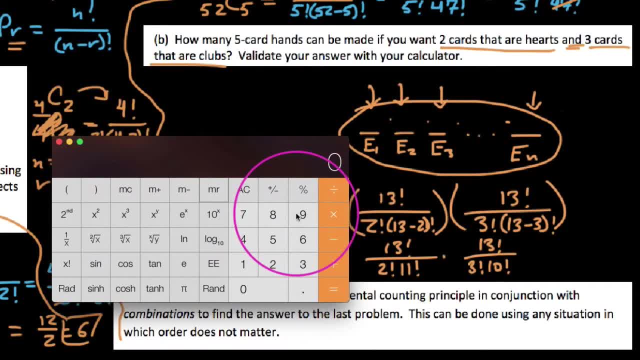 as a matter of fact, going to have to deal with decimals again, but in this instance we could say 13 factorial times 13 factorial on top. we're going to get a very large number here. so that's our top value here, and then we're going.